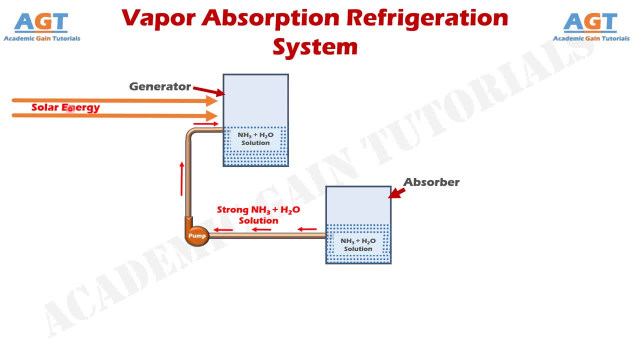 here. heat is produced inside this generator using the solar energy supply to it, And when heat is applied to this solution, both ammonia and water from this ammonia water solution turns into vapor inside this generator. We also have an analyzer inside this generator. 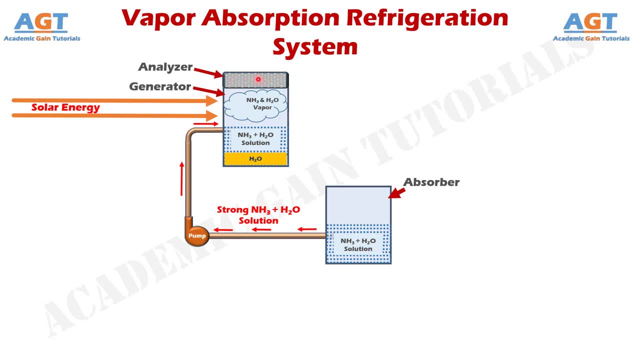 When this vapor of ammonia and water is passed through this analyzer, the analyzer sends the water vapor back to this generator. Not only does it generate heat, but no water vapor by the generator itself, This ooksum, and it only lets the ammonia vapor to pass through then from this generator. 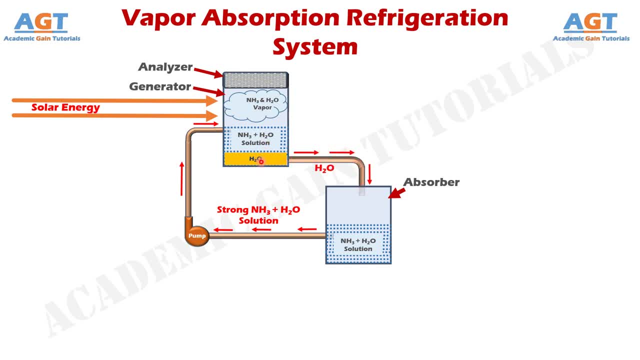 the residue of water vapor accumulated here will be passed back to the absorber again through this connecting pipe. now, even after passing through the analyzer, there will be some proportion of water vapor mixed with this ammonia vapor. so here we have a rectifier. this rectifier can also be called a separator. 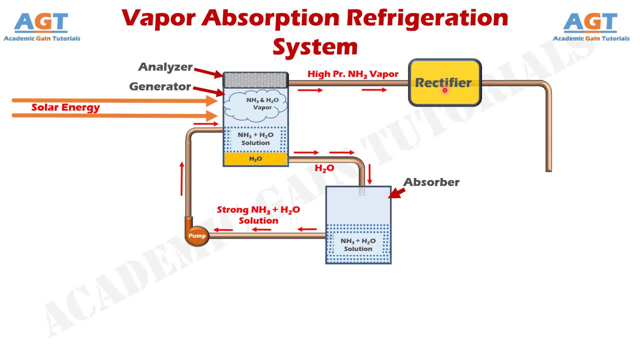 because it separates the rest of the limited amount of water vapor present inside this ammonia vapor through the exchange of heat. so through the exchange of heat this rectifier will convert the water vapor into liquid form and separate it from ammonia vapor. then this separated liquid water is passed. 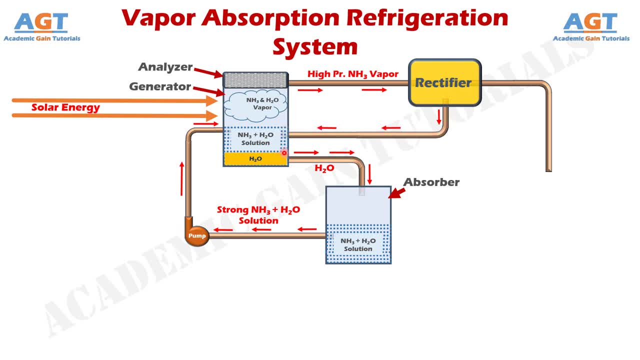 back to the generator. from there it will ultimately reach the absorber. now, after separating the water vapor here, we have obtained pure ammonia vapor. but actually this is not a 100% vapor state of ammonia, because when heat exchange occurred inside the water vapor, the vapor vapor will be separated from the 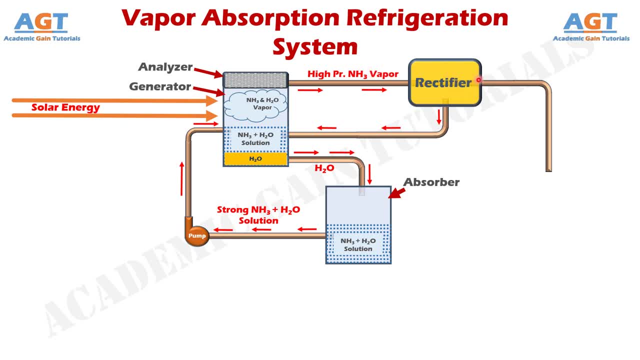 rectifier. the ammonia vapor has also converted into partial liquid ammonia. so this pure ammonia in the partial liquid form will leave the rectifier and enter the condenser through this connecting pipe. here we have a condenser when high-temperature, high-pressure partial liquid ammonia vapor enters this cold. 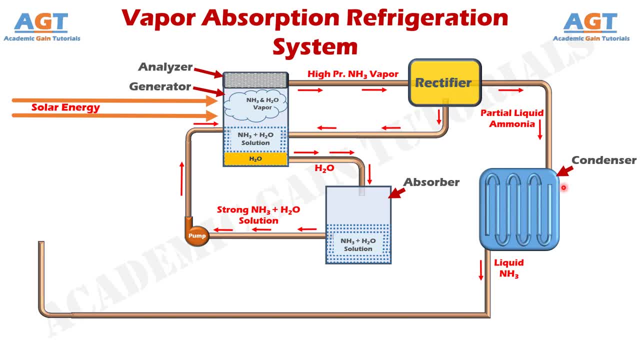 condenser, then the condenser absorbs the heat from the partial liquid ammonia vapor and completely converts it into liquid. this condenser can be water-cooled or cooled by any other system, and this condenser can also be used as a condenser for the solid bathtub in an external source, which will liberate the latent heat of. 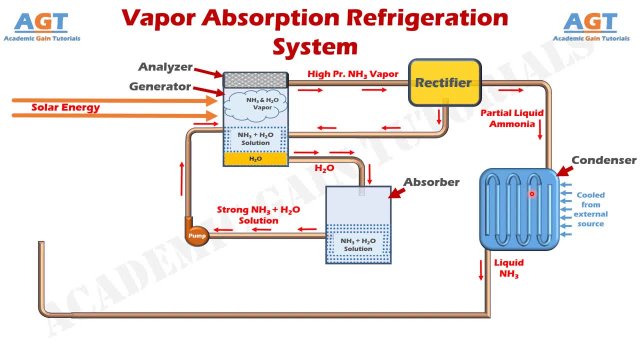 this vapor coming into the condenser and thus condensing keeps happening. now here we have an expansion valve. after condensation, liquid ammonia will leave the dispenser and pass through this expansion valve. now this high-pressure liquid ammonia coming from the condenser will be expanded inside this expansion.